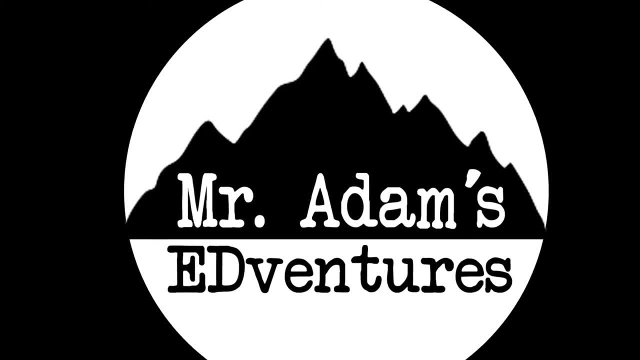 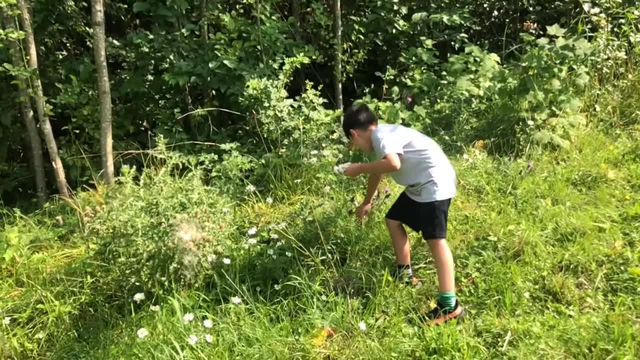 Hey kids, Mr Adam, here and today we're going to show you how to make beautiful sun catchers Most of the supplies you can find right in your own backyard. We started off by searching our yard for supplies we could use in our sun catchers. 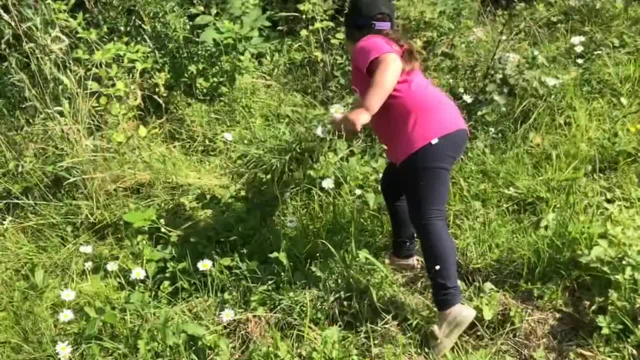 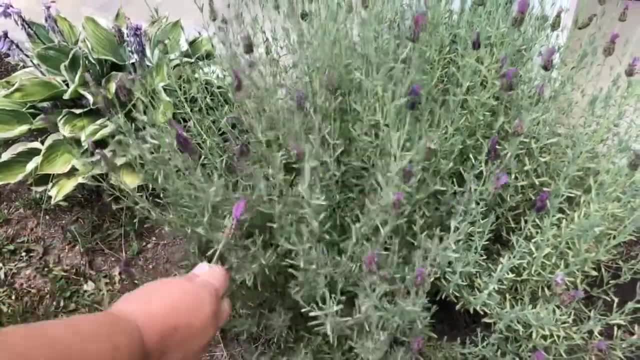 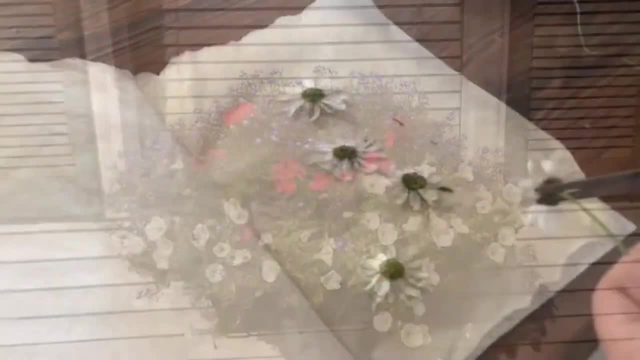 We picked different flowers and plants that we thought would look nice. We picked daisies, buttercups, ferns and lavender. Maybe we should pick mom's flowers? Hmm, better not. In order to make our sun catchers last longer, we decided to press and dry our flowers using the microwave. 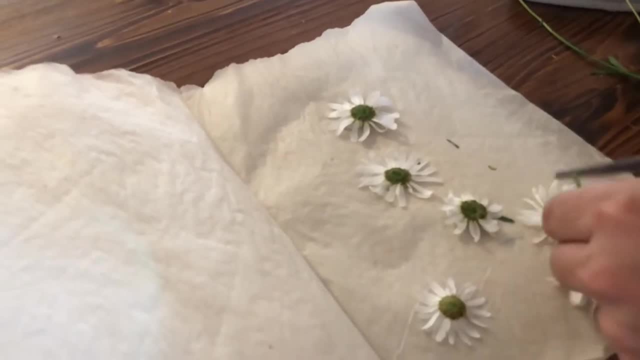 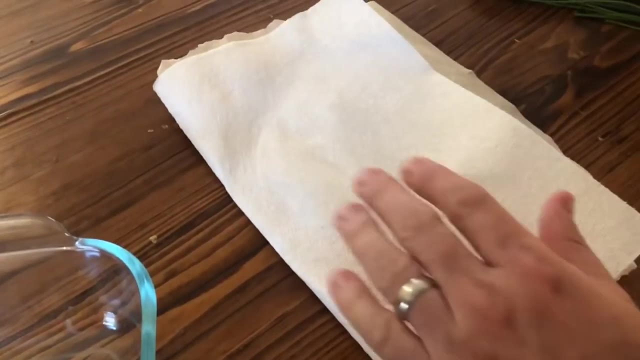 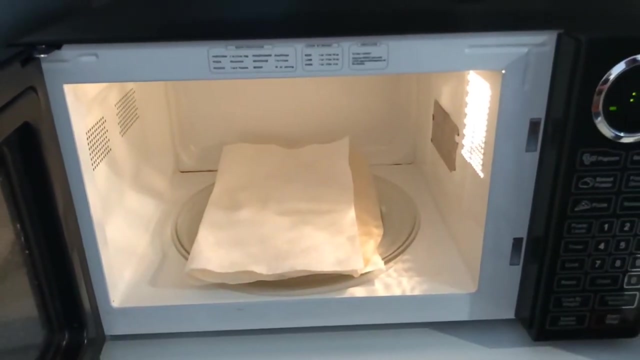 We started by trimming our flowers and plants to the size we wanted. We then placed the flowers between parchment paper and wrapped the parchment paper with paper towel. This helps absorb the moisture from the plants. We then put this in the microwave and placed a heavy dish on top to make sure the flowers stayed flat. 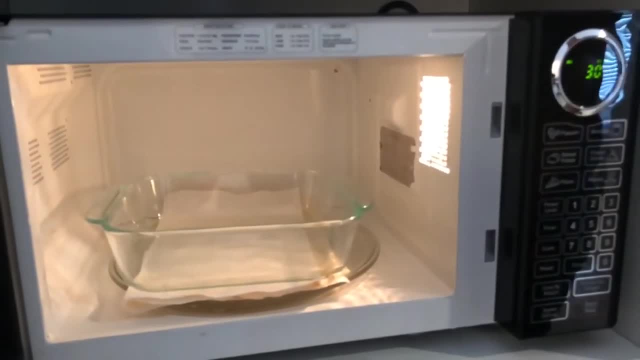 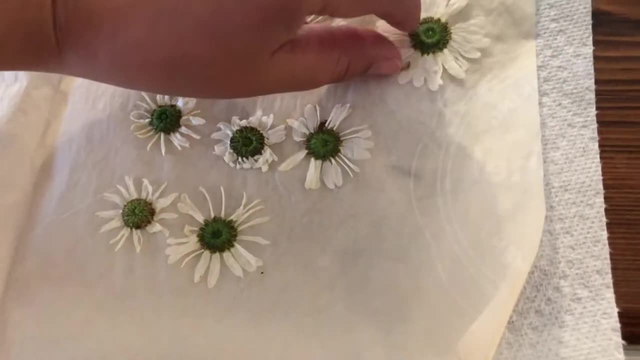 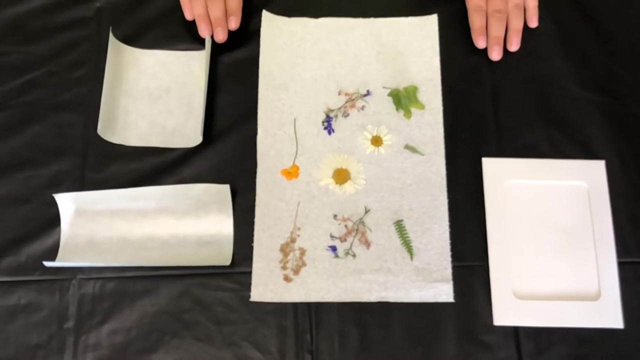 Cook the flowers for about 60 seconds, but only for 30 seconds at a time. This will prevent the flowers from burning. After 60 seconds, the flowers should be dry to the touch but not falling apart. We cut two pieces of clear contact paper the same size for this next part. 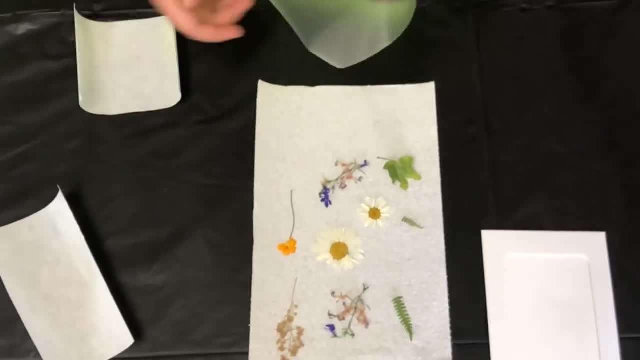 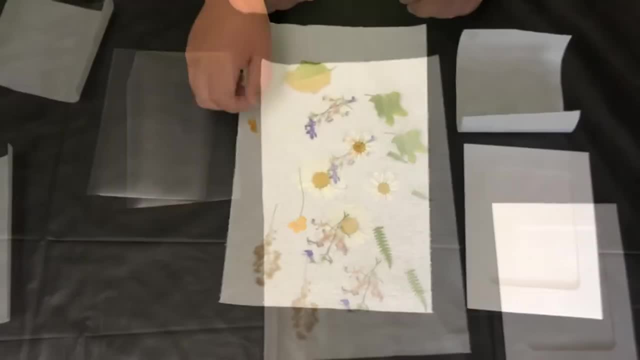 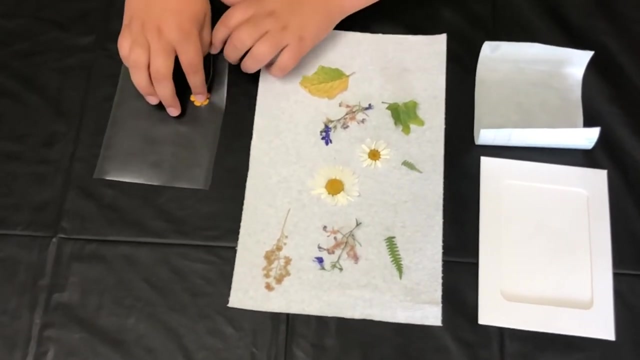 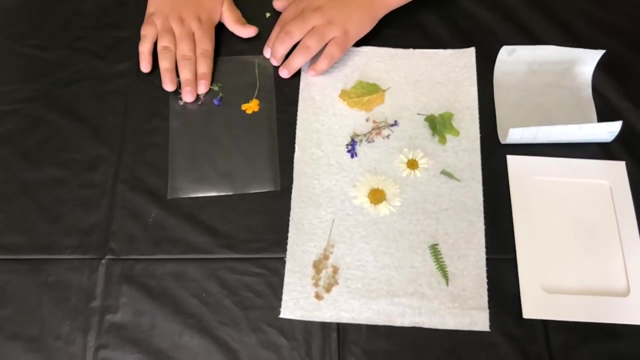 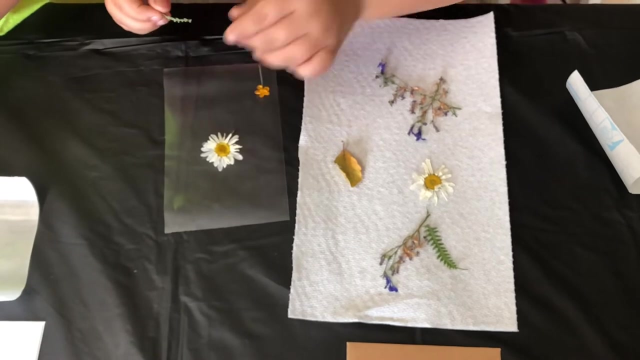 We started by peeling one of our contact papers and placing it sticky side up on the table. We then carefully placed our flowers on the sticky side of the contact paper. Remember there is no right or wrong spot to place your flowers. Don't forget to place your flowers on the sticky side of the contact paper. 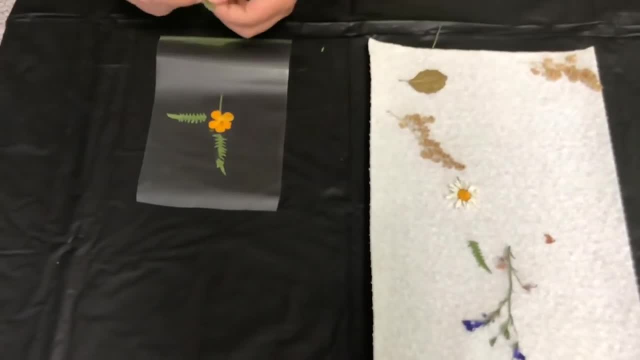 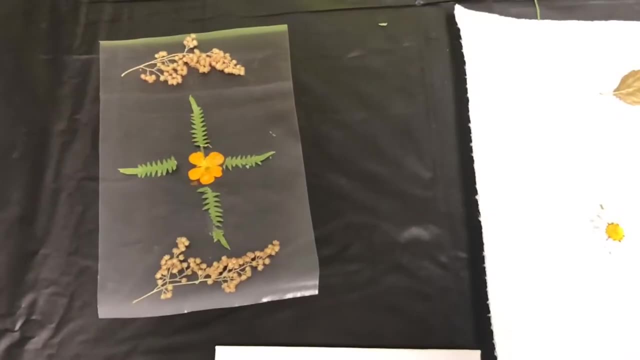 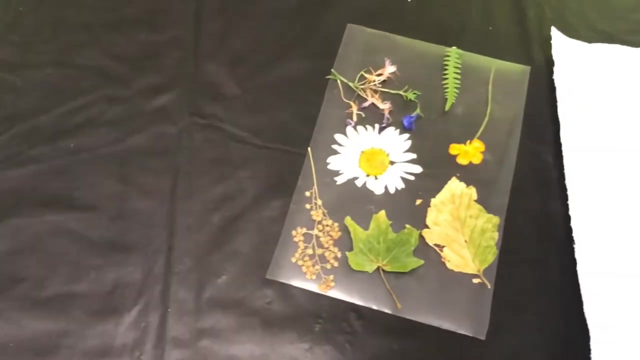 We then carefully pushed the contact paper between the closely attached flowery parts of the flower. After this step, we pressed the flower in place. We then applied the dye to the flowers, but did not use any of it. We then offed the flowers for the wavy sides.